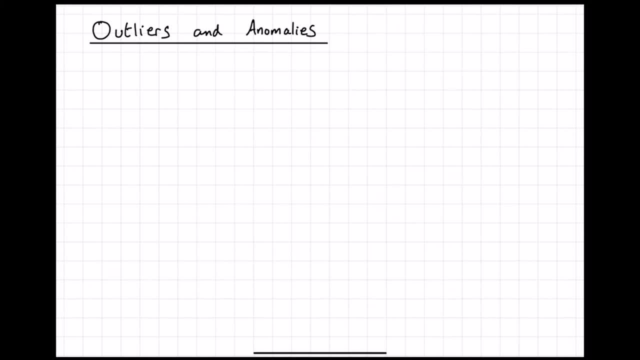 and that's not really lying inside the pattern of your overall data. So imagine I had like a bunch of ages, right, let's say I had um. well, let's say I was just um checking the heights of different people. So let's say I'd have someone who's 150 centimeters tall, 160,, 180, let's say someone was 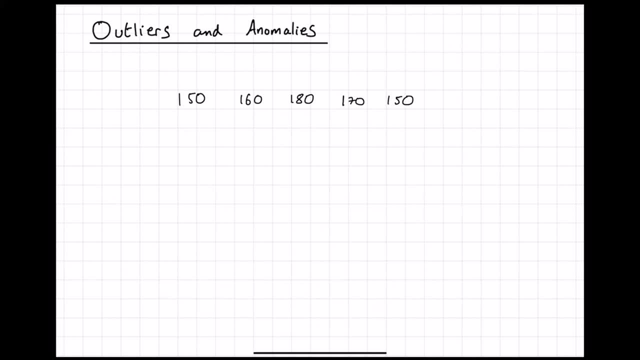 170, 150 and so on, and then suddenly I had a value which was like 230.. So in general these values are quite close to each other, but then this one seems particularly larger than the rest. So you can see, the biggest difference between all of these numbers, between large and small, is probably 180,. 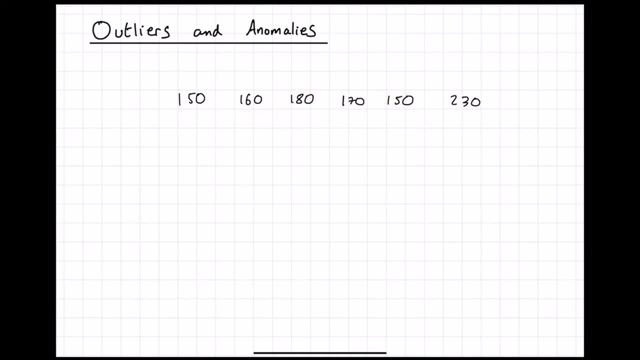 150 here, so there's only a spread of about 30, but this one over here is much, much larger. So, depending on how large this is, if it's too large, then in different cases you would call this an anomaly. So, for example, let's: 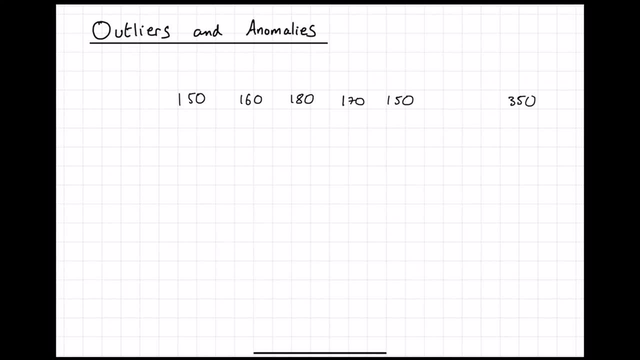 add another one who's 350 instead of 230.. Well, in this case, what would end up happening is we'd say, well, this one probably is an anomaly because it's so far from the other piece of data. So essentially, that's um, and also, yeah, we'd consider that as an outlier, basically. So that's essentially what. 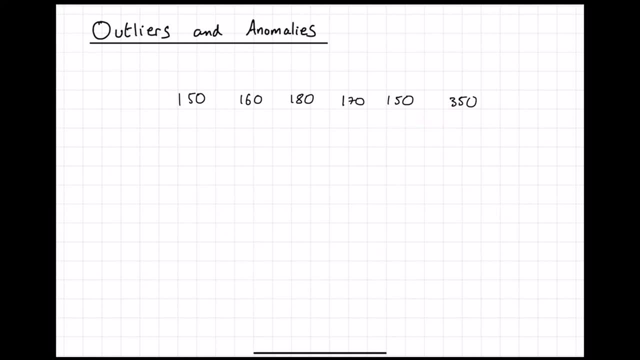 we've got here Now. sometimes you might have outliers from your data, but it doesn't necessarily mean that it's not part of your data. Sometimes it might genuinely be that you actually have got someone who's 350, but we'll talk a little bit more about that after we've discussed the definition. 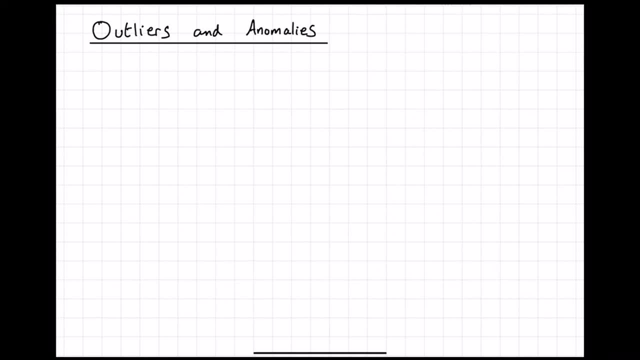 for an outlier, So hopefully that makes sense. So essentially you have a pattern of data and if something is either too low or too high compared to that data, then you call it an outlier and sometimes if you consider this data point which is outside, or this one over here to be wrong, you 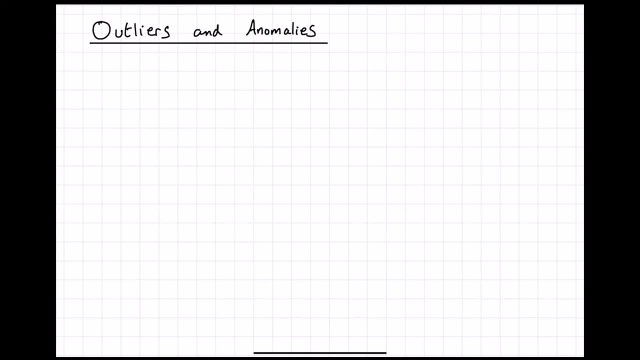 normally call that an anomaly and you get rid of it. So let's talk about the statistical definition of what an outlier is. So there's different ways you can define it, depending on different values, but the way that we do it in stats is usually if you take your third quartile and you add on k, lots of the interquartile range, so that's q3. 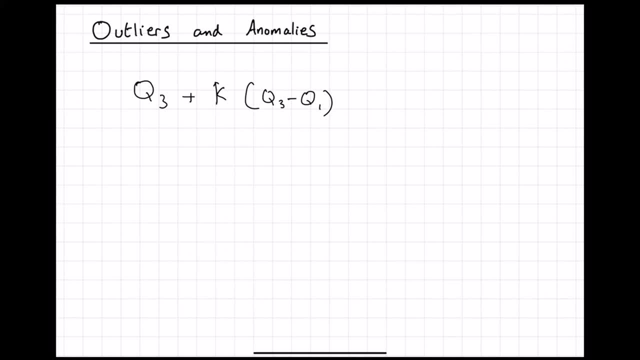 minus q1, then anything which is going to be more than that is considered an outlier, and anything is. if you take your lower quartile and you take away k lots of the interquartile range, So that's q3 minus q1.. k lots of the interquartile range, That's also considered an anomaly. So just to explain to you, 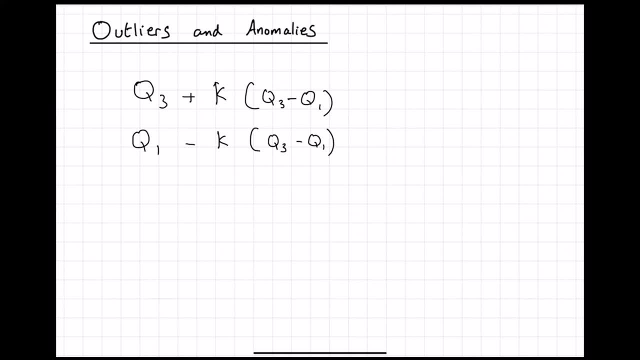 what this looks like on a graph is something like this: So let's say we have a box plot like that, or before that, actually, let's actually have an even easier example. Let's say I've got a line like that: This is q3, or this is actually q1.. This is q3.. This is q2.. So what I'm trying to say 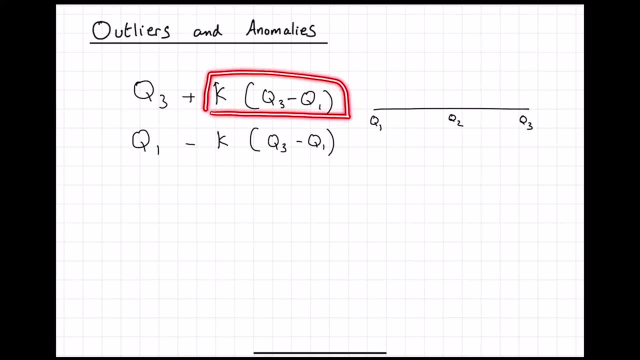 is that anything which is k times the interquartile range more than q3 is an anomaly. So I have a tolerance of this much. Anything which is within that is okay, but anything which is more than that would not be good. Same thing from q1.. The only difference is the sum going down, So we care about. 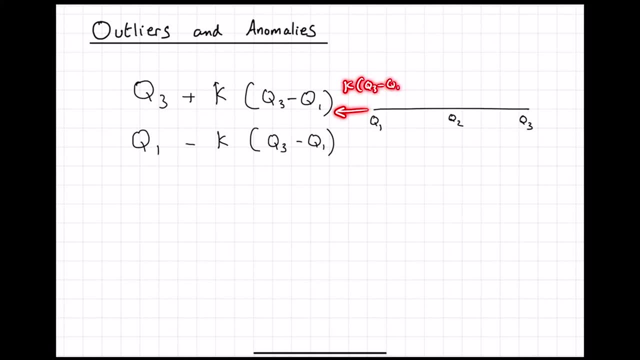 minus lots of that. So kq3 minus q1 lots. Anything over here is okay, but anything which is beyond that is bad. So basically we have a tolerance level between the two. So anything like that would be considered an outlier. And sometimes, just coming back to what- 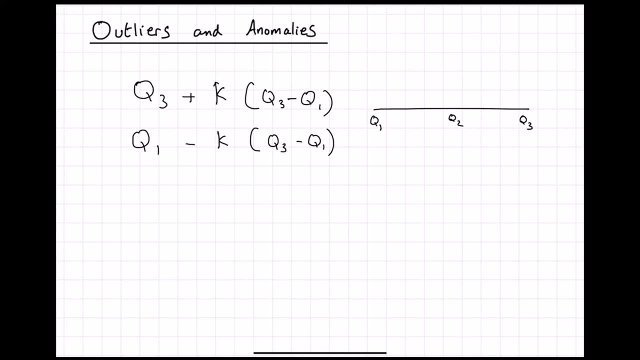 anomalies are. there's sometimes that we find our data has outliers. So let's say: this is my data and I found that this is everything, which is fine, and then these are the points, let's say, which happen to classify as outliers. Now, sometimes what happens is that if I were to include these, 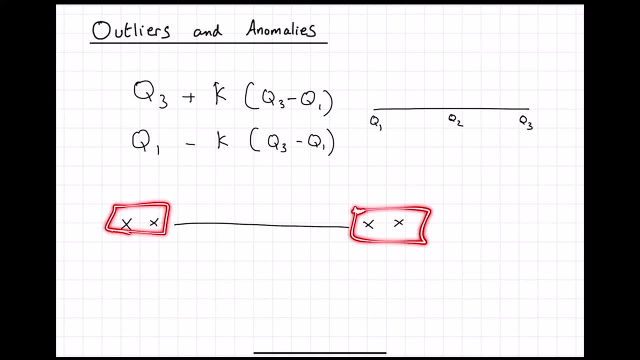 since they're outliers, they might skew my data or they might give me misleading results. So sometimes your outliers can be considered anomalies, and the ones which you get rid of, or data points which make your outcome misleading, they're called anomalies and you tend to get rid of them. So you wouldn't actually include any of these if you're doing that, But you have to be. 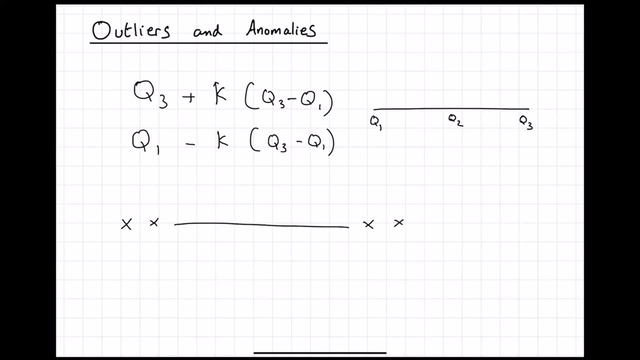 careful as to what actually is an anomaly, because sometimes outliers are genuine values which could be correct. So you know, if I was doing heights, there really could be someone who's like 230, let's say So. sometimes you don't want to take it out and that depends on. 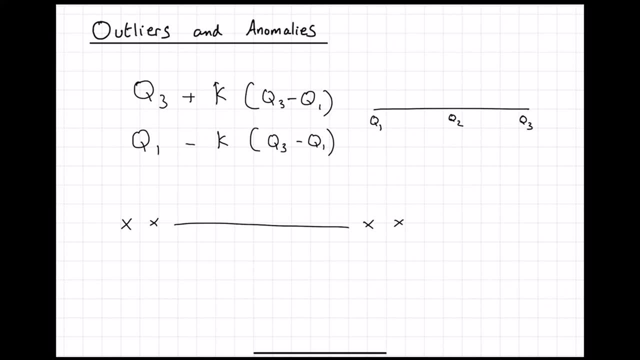 what kind of experiment you're doing or what you're trying to figure out. That's like one of the questions you have to solve in stats, But in A-levels you won't have to worry about that. They'll usually tell you what's considered an outlier and whether to get rid of it or not. 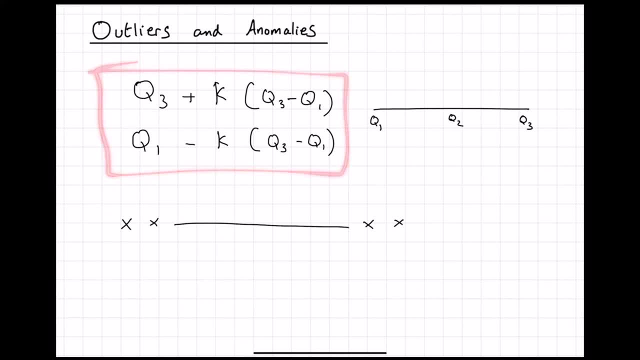 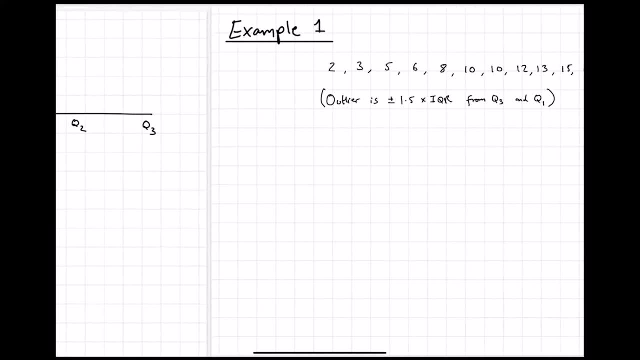 So since we've done all this talking about this equation here, it would probably be a good idea to go through an example of actually how we use this equation. So, moving on, let's take a look at our first example. So here we have a set of numbers, So let's see how many numbers we actually 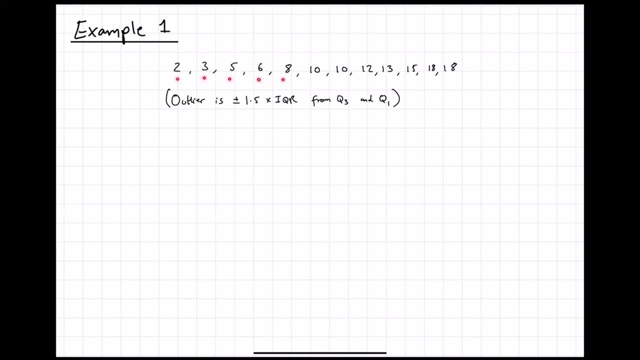 have in total. first, We've got one, two, three, four, five, six, seven, eight, nine, ten, eleven, twelve numbers in total. So let's just write that down. We've got twelve numbers That'll be useful to know, And basically we're going to be given. 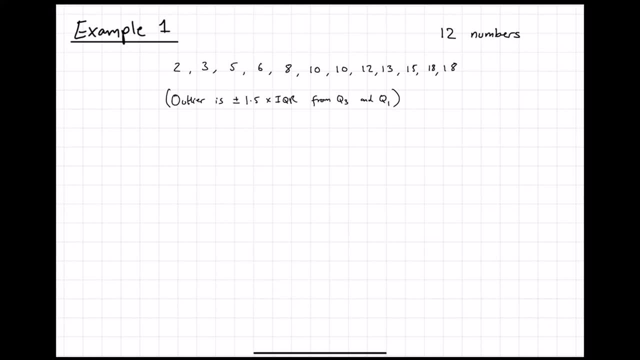 what the outliers are, And I know that last time we wrote the equation as being k, lots of q3 minus q1.. The thing is, k will normally be given to you in your A-levels. You don't actually have to work out a value of k, So you're normally going to be given that. So let's say we're given the. 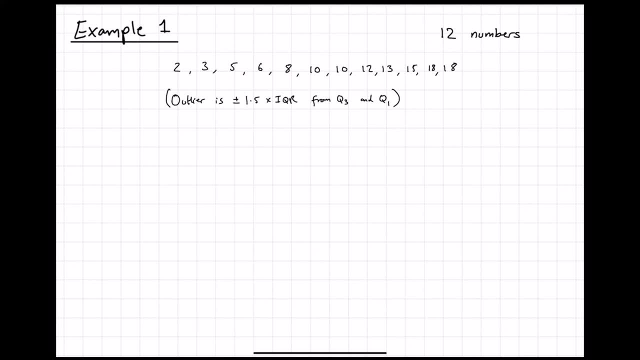 set of numbers and the definition is that here the outlier is plus or minus 1.5 times integral to our range. I'm just using that because that's the same thing as q3 minus q1.. I can't even bother to write that out- And from q3 and q1. So it's just basically saying it's these two here. 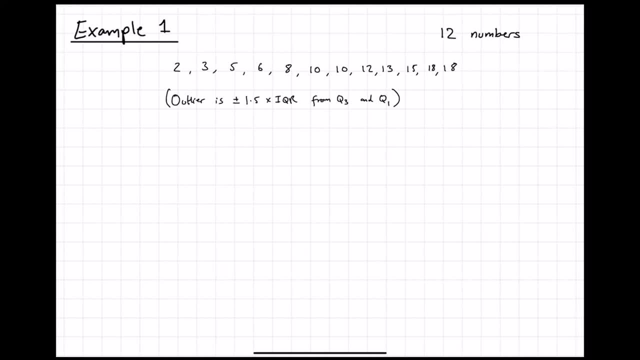 So let's take a look at what our answer should be for this. So how do we start this? Well, the first thing you want to do is you want to figure out what your q3 and q1 values actually are for this equation, And to do that, we need to figure out how many data points you have in total, which is 12.. 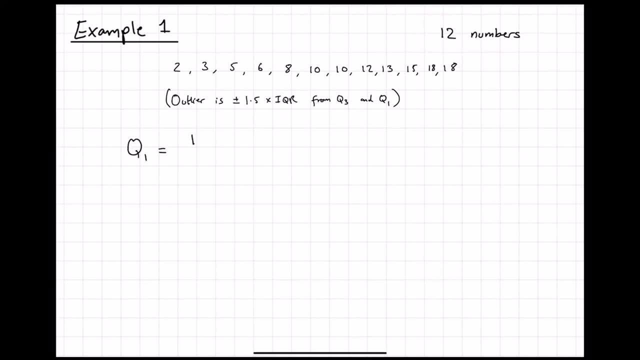 Great. So let's do q1 first. So we now have 12 data points and we know to find the lower quartile divide that by 4, which gives us the third value. So the third value, if you just look along. 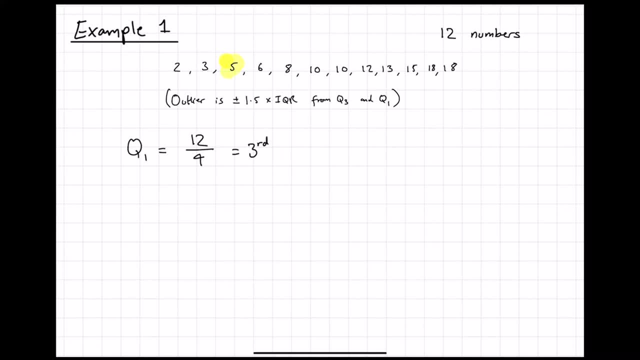 would be number 5 over here. That's our third value. So that means 5 is our lower quartile. Now let's find the upper quartile. So this will be 12.. Times 3 divided by 4, which is 36 divided by 4,, which is the ninth number, So the ninth number 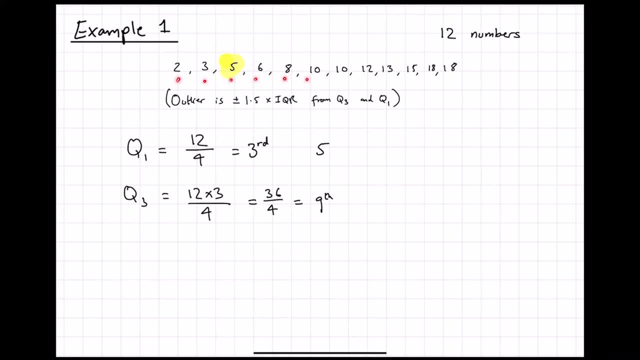 along would be 1, 2,, 3,, 4, 5,, 6,, 7,, 8, 9.. That's 13.. So let's mark that down as our upper quartile. Cool, So now we have our two quartiles. Now, according to our equation, what we said. 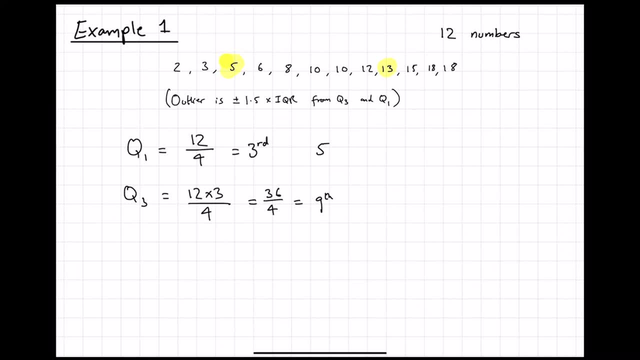 was, the outliers were anything which were plus or minus 1.5 times the interquartile range. So let's do that again. For anything to be an outlier from q1, it has to be 1.5 times the interquartile range. 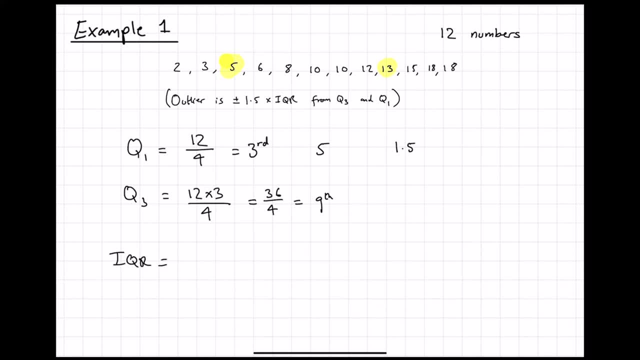 which we know that now We can write interquartile range as being the ninth number was 13.. So interquartile range is 13 minus 5, which gives us 8.. So anything which is 1.5 times 8,. 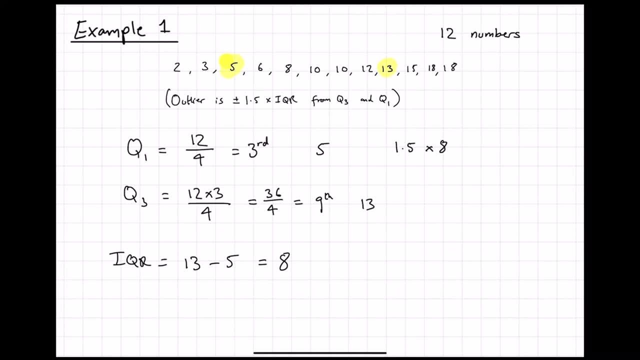 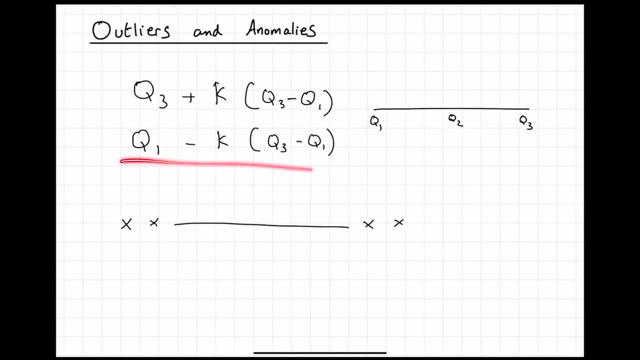 and then our lower quartile is 1.. So we do 5 minus 1.5 times 8, just following from q1.. This equation over here, This over here, we found that to be 5.. That's given as 1.5.. And we just. 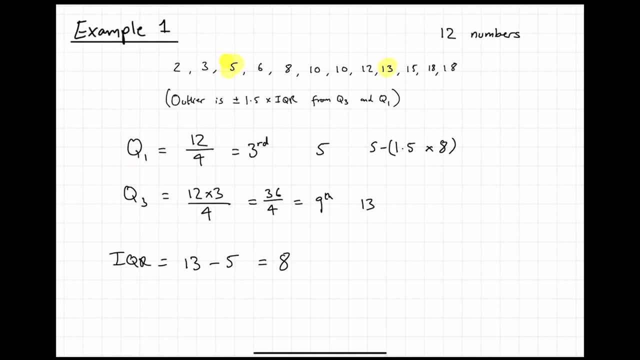 found the interquartile range of this whole thing was 8.. So, coming back to here, that's what we get. So if we were to solve that, this goes to 5 minus 8 times 1.5 is 12.. So our lower quartile gives us: 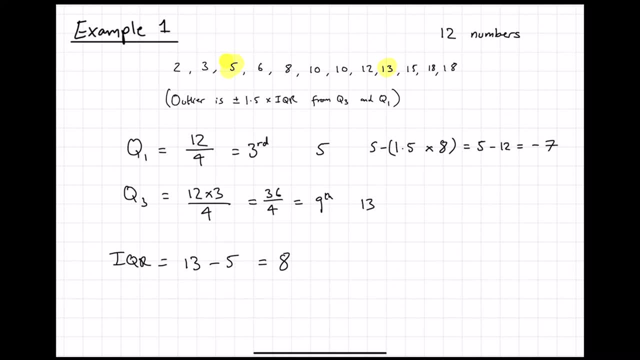 a number of minus 7.. So if you had any numbers which are minus 7, then those would be be or anything less than minus 7, that would be an outlier. But you can see, in this data we don't actually have anything which is less than minus 7, which is completely fine That. 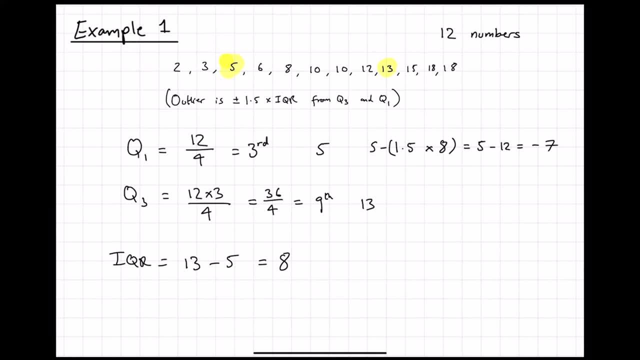 means we have no outliers on the left-hand side over here. Let's try that for the other side, on this upper one over here. So the upper quartile is 13.. So 13 plus 1.5 times 8 gives us 13 plus 12, which is 25.. So here we can see that nothing is more than 25.. So actually, 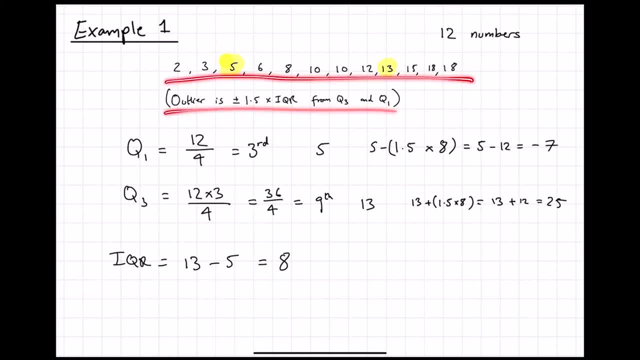 there are no outliers in the data set. Everything is fine in this data set according to this definition. Let's say I had randomly added on a number which is like 48. What I might have ended up doing is it would change your interquartile range and the other values. 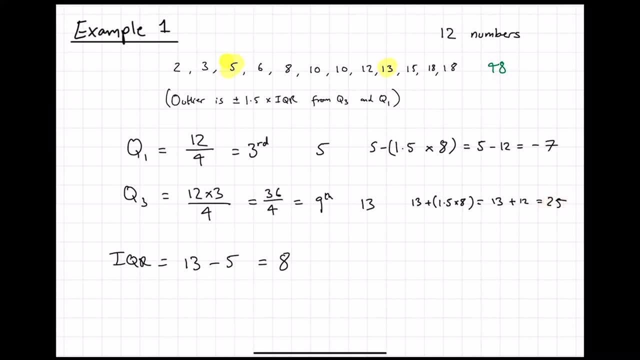 but probably the value which is the upper one here wouldn't be 25.. It could have been something like 27 maybe, But then what ends up happening is This number would have fell outside it, So in this case we have no outliers but anything. 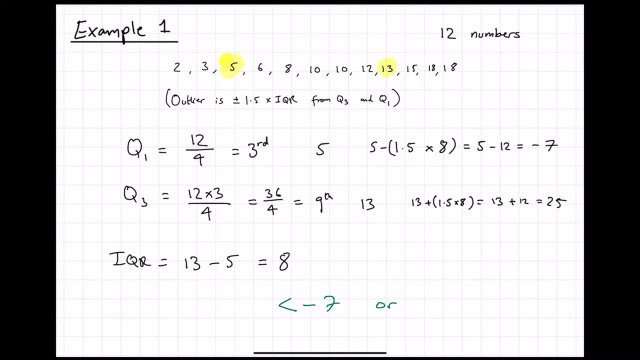 which is less than 7 or more than 25 is considered an outlier, And you just have to check if there are any outliers in there. So that's pretty much all you actually have to do for a question like that. So these are quite simple to follow. It's just essentially: you've got. 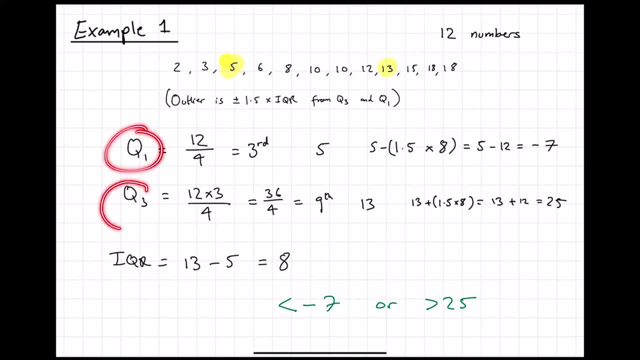 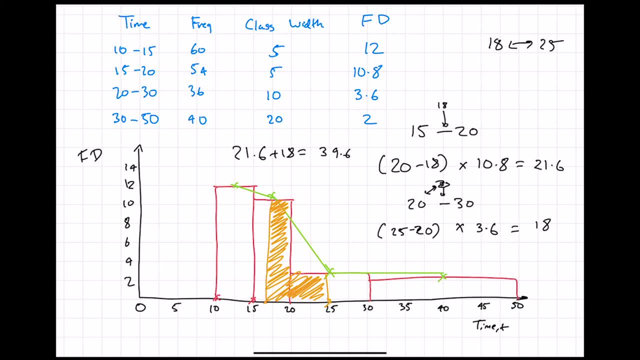 39.6 is the value, so the estimate would be roughly 39.6 students and you can say, if you round that up, is roughly 40 students is what you should have. but in terms of student wise or in terms of numbers, you can say that this is the answer of the estimate that we've given. obviously, 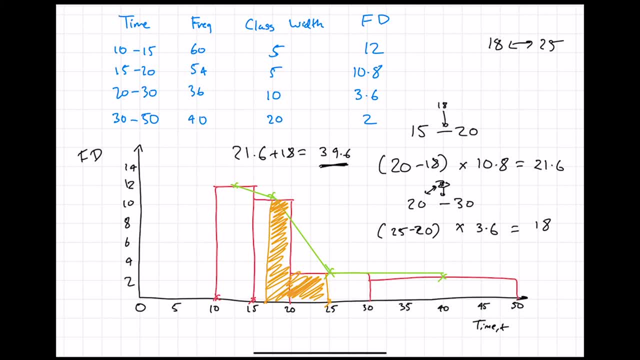 you can't have that many students, so you actually should be something like either 39 or 40. but that's how you figure out. so what did we actually do? first, we figured out that this is the times we want to go in between. so which class does 18 fall into and which class is 25 fall into? we found it. 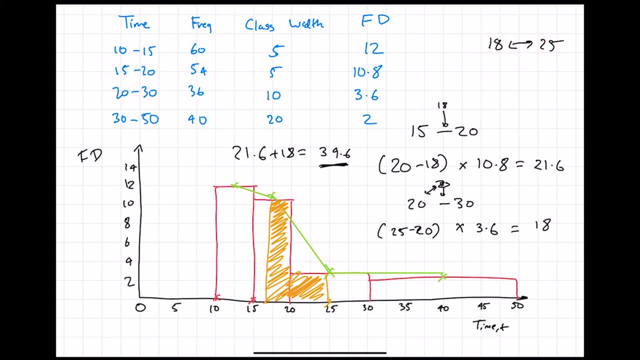 fell into this class and this class, then we want to say: if it's 18, well it's. this is 15 to 20 and 18 is like somewhere over here. so we need to find out how far 18 is from 20, and same for the other. 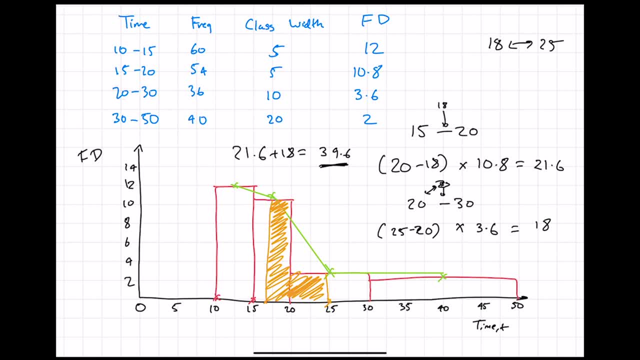 one, this is 25. how far is 25 from 20? so when you find out how far they are, so this is 20 minus 18, so it's 2, and this is 25 minus 20. you multiply with them by their respective frequency densities. 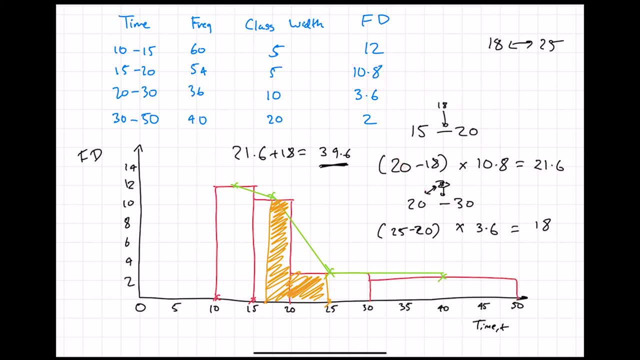 and then you get your two answers which you add up and that gives you your final frequency. so i hope that wasn't too bad, and then we can go through some more examples in another video of how to do this kind of question. so once you've done that, there's another type of question you can. 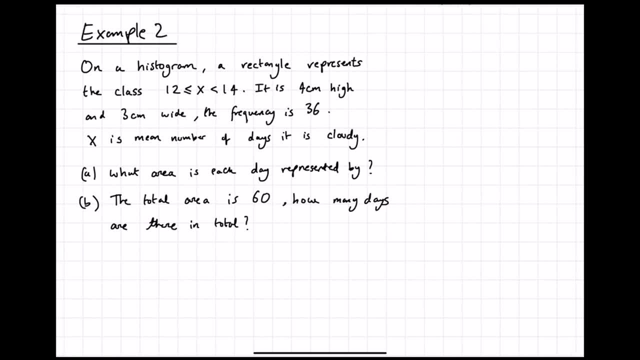 so this is a question that you can take a look at. so it's quite a bit to read, so let's go through it together. so it says on a histogram: a rectangle represents the class 12 to 14. it's four centimeters high, three centimeters wide and the frequency it represents is 36. 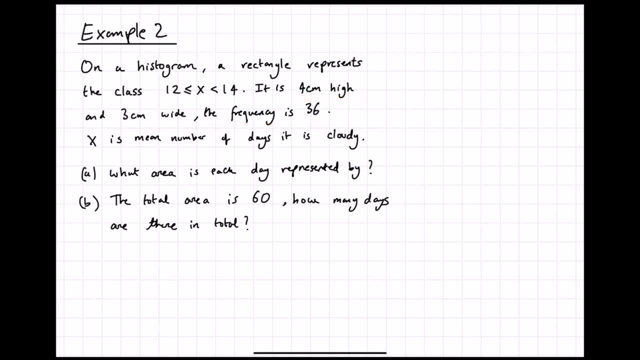 and x is the mean number of days that's cloudy. so let's say, maybe the number of days is cloudy in a year, that's a mean number of days in a city. so what area is each day represented by? so, just so you know, what's happening is we have a rectangle from 12 to 14, which is three centimeters wide. 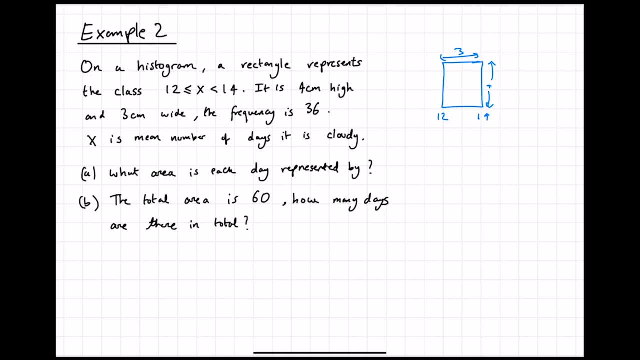 and four centimeters high and it represents a total frequency of 36, so the frequency represents is 36. now, this is a rectangle which is part of a whole histogram set, so this is actually what the whole thing might look like, and it's just talking about this one. 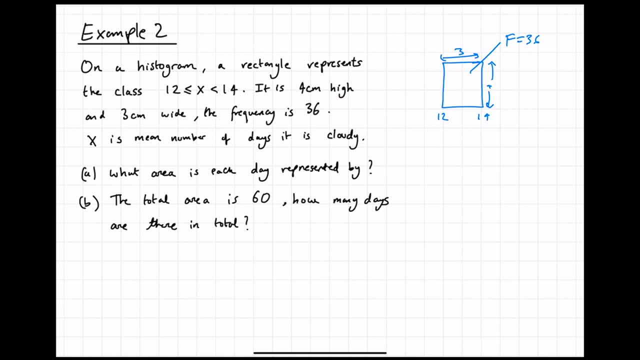 histogram, square or rectangle that we've got here. so the first question is quite easy: it says what area is each here represented by, and to do this, what you have to do first is you find the area of the bar, which is 3 times 4, which is equal to 12, and this area of 12 is representing 36 as a frequency. 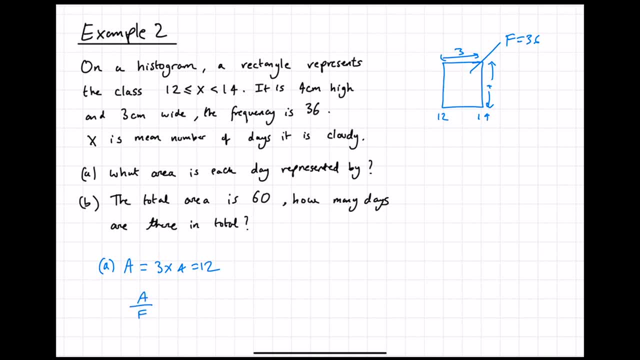 so you just say the area divided by the frequency is what you want. so the area divided frequency is 36, actually 36 on the area. the area is 12 and this area of 12 represents 36 people. so the frequency density is one third, or 0.33 centimeters squared, and that's what each day is represented by. 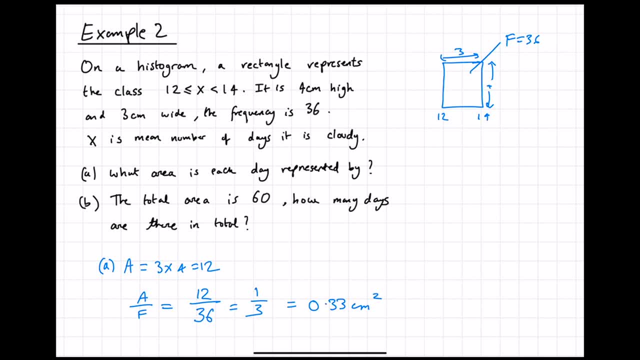 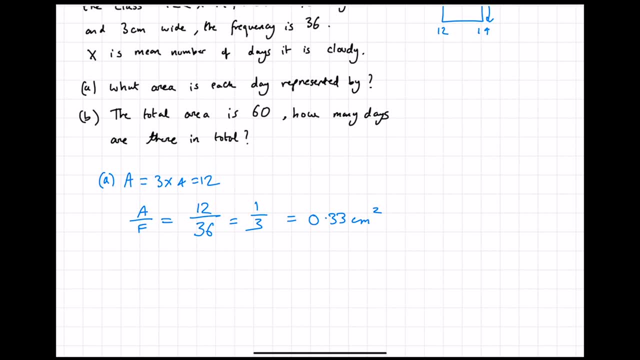 that's what each day is represented by for the area, and then, quite simply, it says: the total area is 60. so if the total area is 60, then how many days are there in total? well, for part b, we know that each day is represented by a total of 60 days. so we know that each day is represented by a total of 60 days. 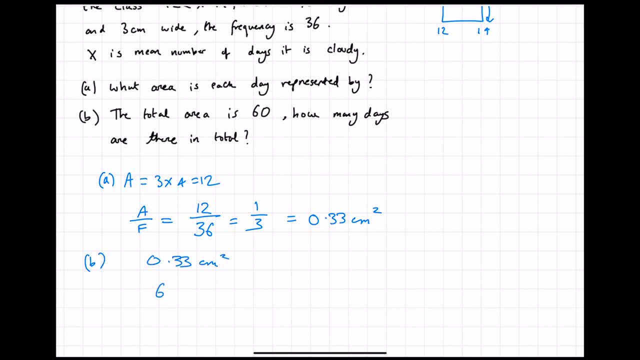 each day is represented by 0.33 centimeters squared. we have 60 centimeters squared. so, quite simply, to find the total number of days, you just divide the two by each other, and i think what might be better is, since we know that actually it's one third, so let's stick to one third. so 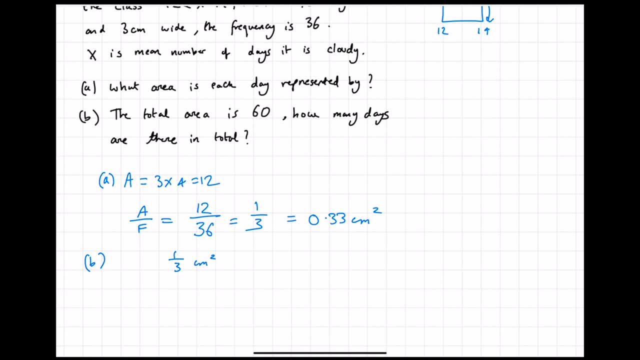 let's say, one third is the area for each day, and we have 60 in total. so 60 divided by a third means that we have 180 days in total, and that's it. we know that, so that's why we're going to do this. 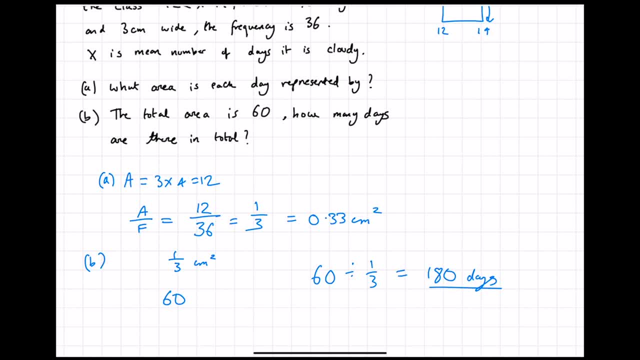 that there's 180 days in total. so these kind of questions are quite simple. if you just follow the area, figure out. if you've got a total number of frequencies, then for that total frequency all you have to do to the area divided by the frequency and it gives you whatever is represented for each. 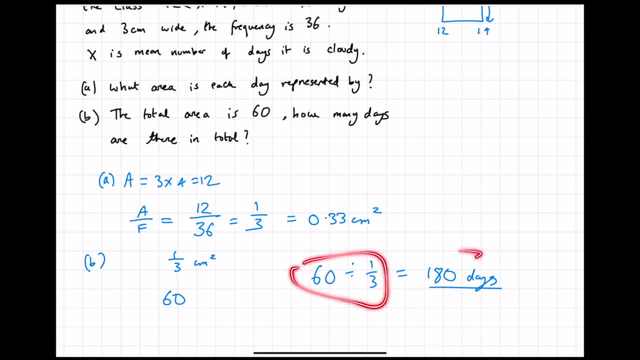 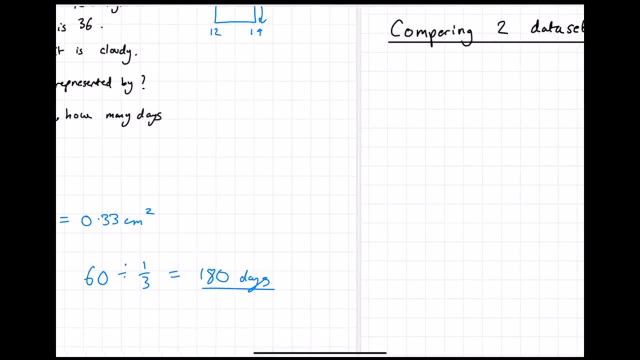 kind of day and then if you have a total area you can just divide it by that and get the total number of days. so this kind of question is quite simple to follow and that's kind of it in terms of representation. the last thing we have in this chapter is comparing two days of sets, which we've 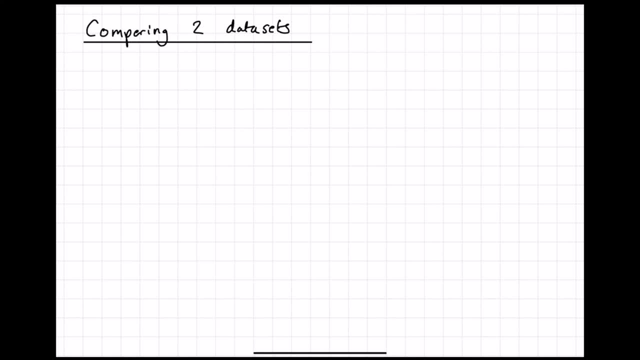 talked about, but we'll just really briefly recap what we said. so there's two things you can do. you can compare the measures of location and we've already done this before because we talked about talk about the, you know, the interquartile range or not that one? sorry, we talked about compare the. 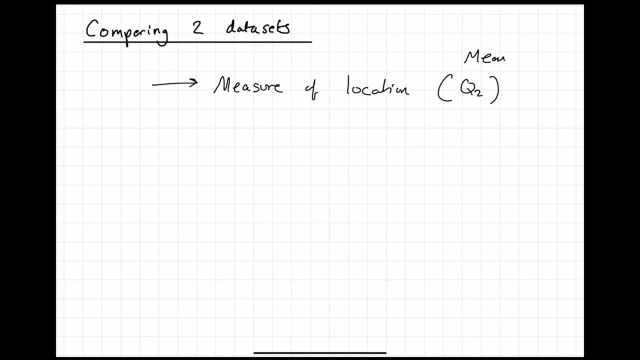 median. so you saw that q2. we might talk about the mean in some questions. you might talk about stuff like that. you might talk about the mode or whatever, and then the other thing you're going to compare is a measure of spread. so that's another thing you want to put. so you might want to put in stuff like you know, the variance. 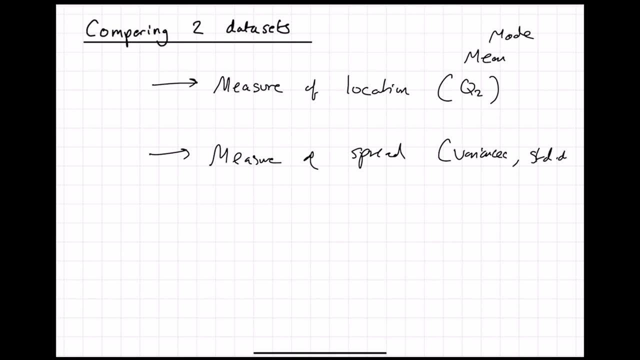 you might want to talk about the standard deviation and so on, but these are the two things you want to compare. you want to compare a measure of location and a measure of spread. so normally when you have a question, you can either compare data using like mean and standard. 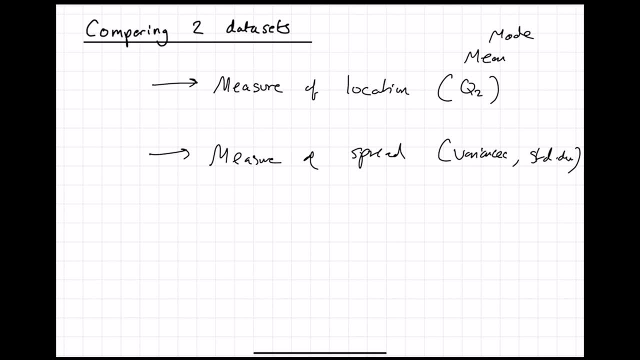 deviation. so usually a measure of location. the standard ones would be: if you have the mean, you would then use a measure of spread, which is the standard deviation, or if you have the other one, that would be, you look at the median and if you have the median, you tend to compare that with the interquartile range.